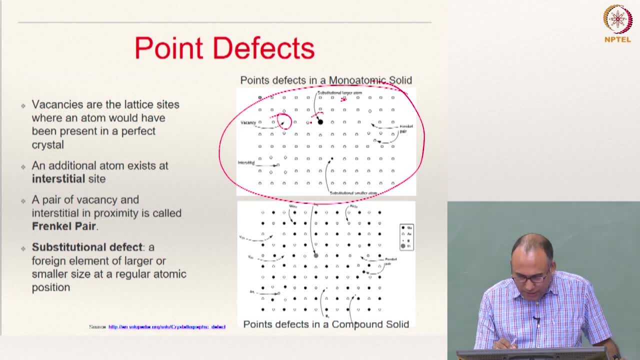 vacancy. And here you see that there should be an atom of this type, but some other foreign atom which is larger than this one is actually coming and sitting is actually substituting for the position of the parent atom. right, It is actually substituting the parent atom. 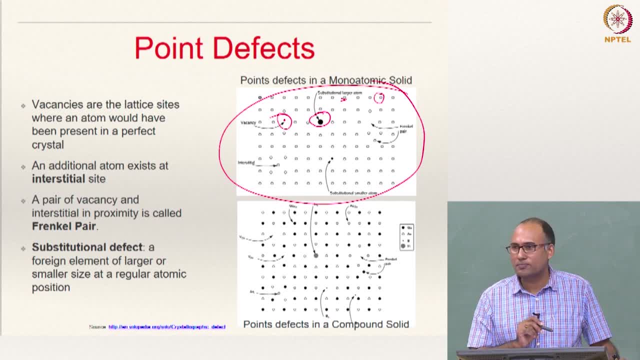 defect, and hence it is called substitutional impurity, substitutional point defect. It is actually substituting for the position And here, if you see, this is actually a- not actually not a lattice side, but this atom actually comes and sits in the interstitial. 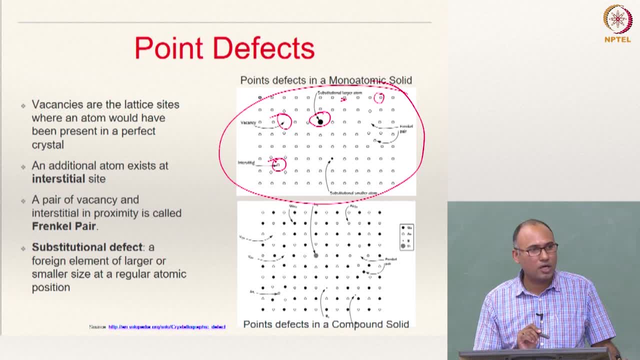 positions available amongst the lattice sides, And hence such a defect is called interstitial point defect. Okay, and now, if you carefully look at it, look here you have a vacancy and very close to that vacancy you have an interstitial right. You have a vacancy here and very close. 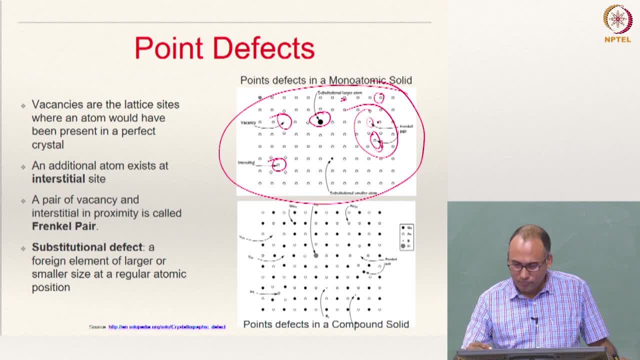 to the vacancy, you have an interstitial, And such a pair is called Frankel pair. It is a one particular kind of a defect. So that means you are having a vacancy, but very close to that vacancy there is an interstitial. 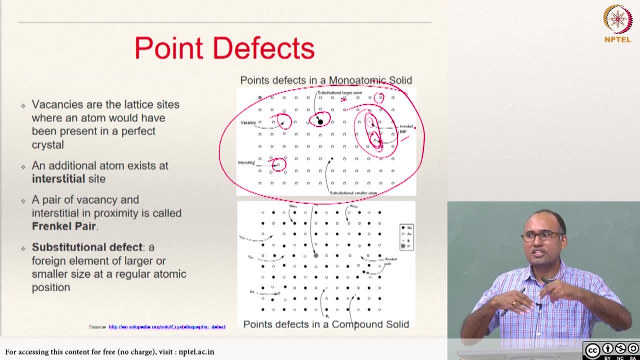 Okay, Thank you. That means it is probably this: the atom which should have been sitting here is actually did not go there and it is hanging around there. So these two, if this guy goes there, it would have become a perfect crystal. And such a pair of defects- point defects are. 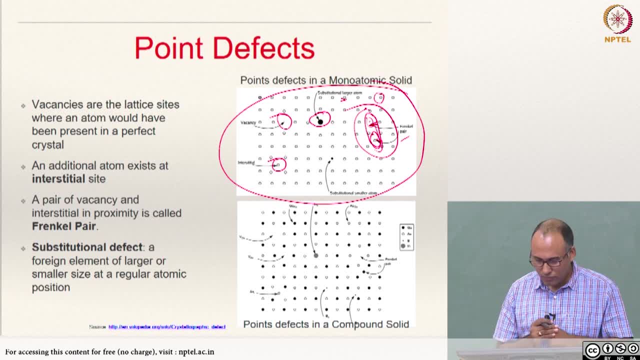 called Frankel pair. Is that clear? Okay, So this is a gallium arsenide system And this here, that what we see is a gallium arsenide system. So the black dots are gallium and this is arsenic right, And then, in that you have impurities of boron and indium right. 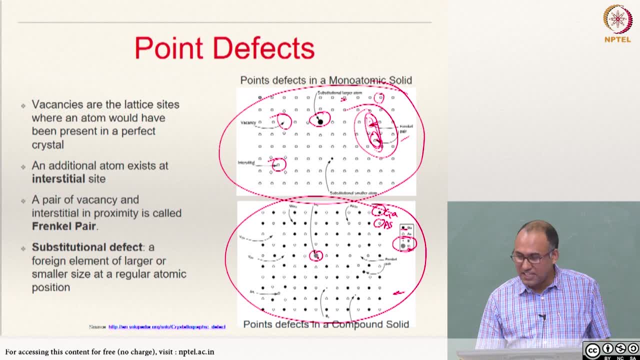 So you have, because the size of indium is larger than all other atoms, usually it forms a substitutional point defect. Okay, Okay, So this is a point defect. So this is a point defect. So this is a point defect. 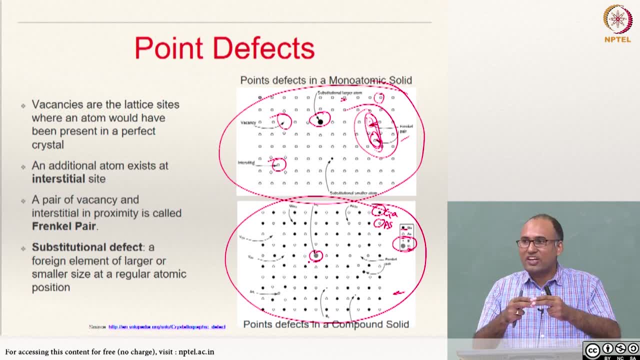 Okay, So this is a point defect. So this is a point defect because the interstitial size will not be having enough space for this boron to go and sit in the interstitial size. And the interstitial size are usually occupied by the impurity atoms, which are smaller. 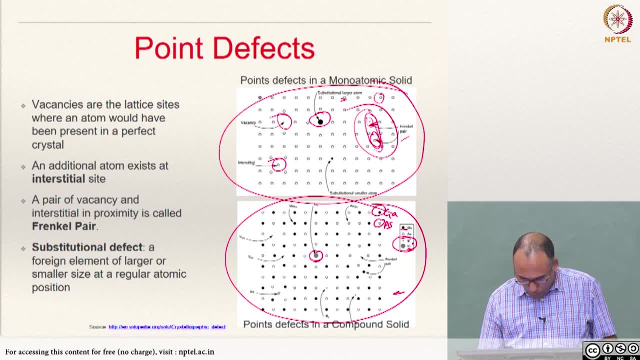 in size compared to the parent atoms. So the boron for instance, if you see here, sometimes it can actually substitute. But there is higher probability for this boron to go and sit near the interstitials because there is free space available. It does not have to. 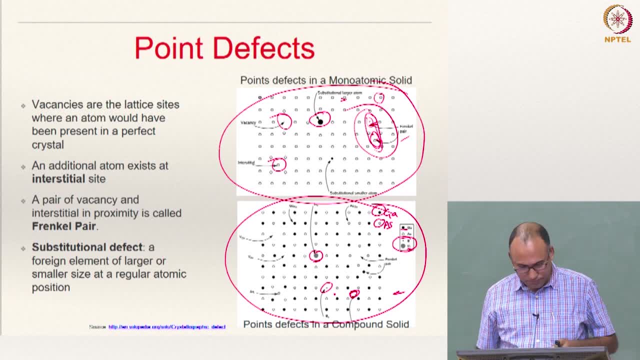 knock off the boron. Okay, So these are the interstitial magnets which are usually occupied, the existing parent atom. ok, So even in inside, even when you are looking at point defects, you have different kinds of point defects, right, depending upon the size of 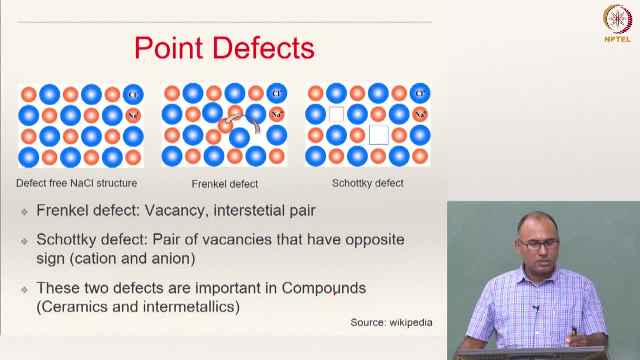 the atoms and so on. ok, So this is for instance, this is NACL structure. This is the perfect guy, defect free. And here you have a Frankel defect. Frankel defect means an interstitial and a vacancy side by side. If you have a vacancy here and you have you. 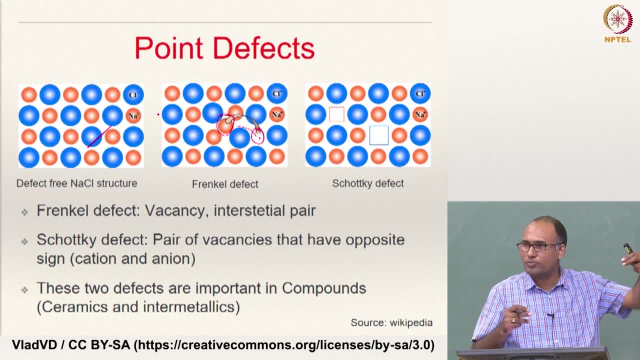 do not have an interstitial here, but from far away, then those two cannot be called as Frankel pair, because they should be close to each other. And there is another kind of defect which is called Schottky defect. What is the Schottky defect? Schottky defect is: 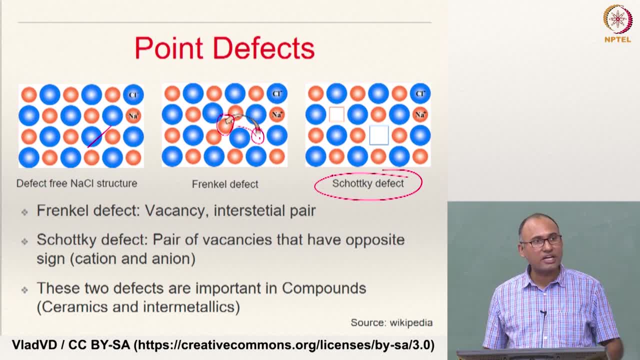 a pair of vacancies that have opposite signs. So it is a pair of vacancies that have opposite signs. That means you have both elements, sodium and chlorine. One is positively charged and one is negatively charged, And you need to have vacancies of these two guys together. So here what should have been there: Sodium. 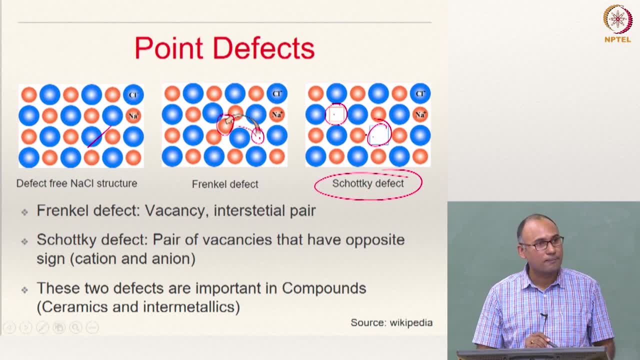 should have been there Here. chlorine should have been there. Both of them are missing, So you have a pair of vacancies which are of opposite side. One is anion and another another is a cation. they are not present in the crystal lattice.